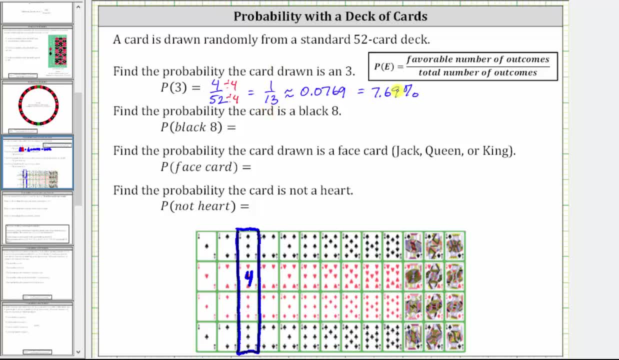 the probability is 1- 13th. These two are rounded. Next we're asked to find the probability of the card is a black eight. So, going back to the deck of cards, here we have the aces, the twos, threes. 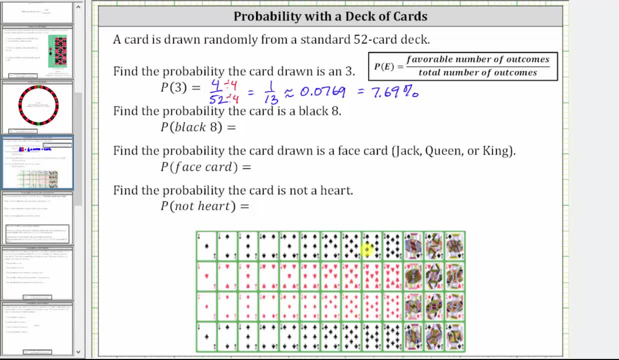 fours, fives, six, sevens and eights. Notice how there are two black eights, There is an eight of spades and there is an eight of clubs. So there are a total of two favorable outcomes out of a total of 52 outcomes. 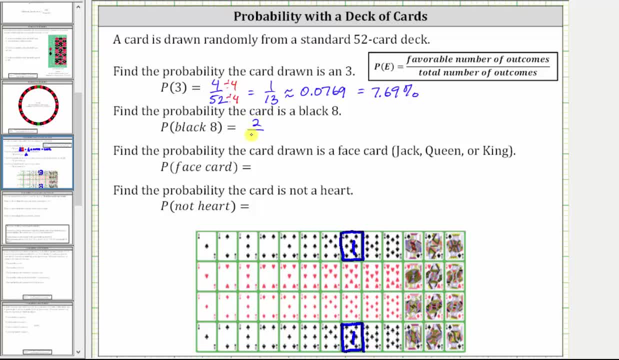 The probability is two. The probability is two divided by 52, or two 52nds. Simplifying: we divide the numerator and denominator by two, which gives us 1, 26th And again let's also show the decimal and percentage. 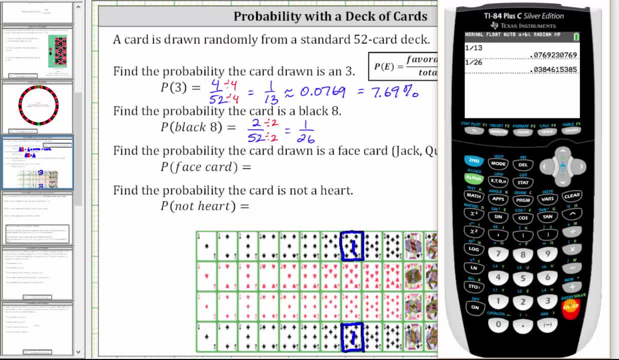 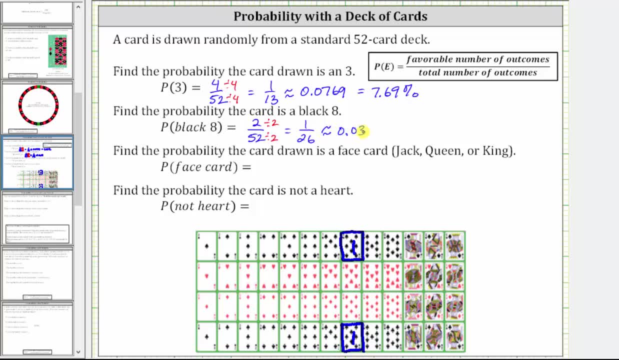 So one divided by 26 to four decimal places is 0.0385, which is 3.8.. 0.0885%. Next we're asked to find the probability of the card. is a face card? Face cards are jacks, queens and kings. 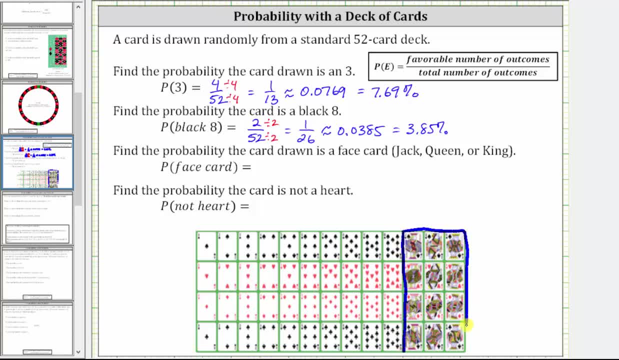 which are these 12 cards here? which means there are 12 favorable outcomes out of a total of 52 outcomes And therefore the probability is 12 52nds or 12 divided by 52.. Simplifying, we divide both 52 and 52. 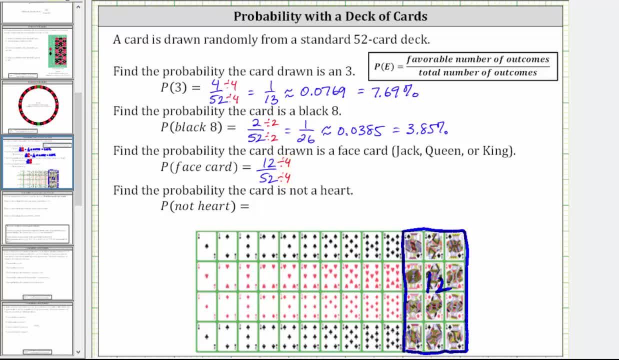 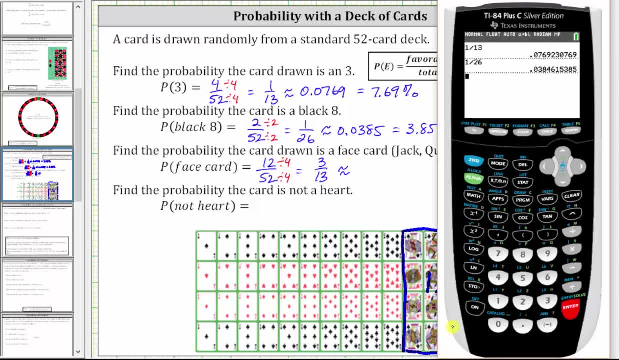 Simplifying: we divide both 52 and 52. We multiply both by four, which gives us 3 13ths, And again show the decimal and percentage. Three divided by 13 to four decimal places is 0.2308,. 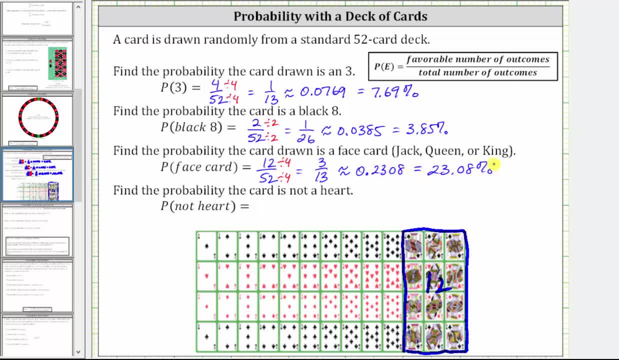 which gives us 23.08%. And for the last example, we're asked to find the probability. the card is not a heart, So the hearts are in this row here and therefore all the other cards would be favorable outcomes. So we have 13 favorable outcomes here with the spades. 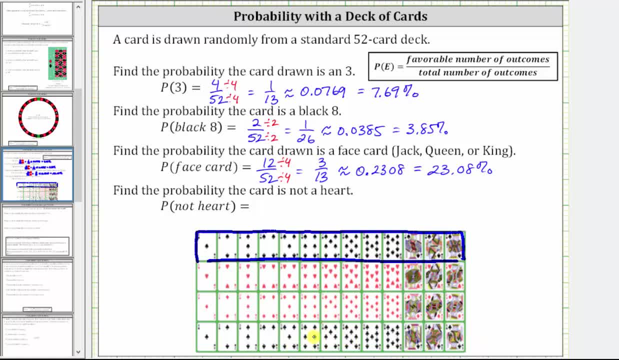 and then 13 favorable outcomes here with the diamonds and 13 more with the clubs, which gives us a total of 26 favorable outcomes here. Again, we have 13 favorable outcomes here, 26 favorable outcomes here, which gives a total of 39 favorable outcomes.